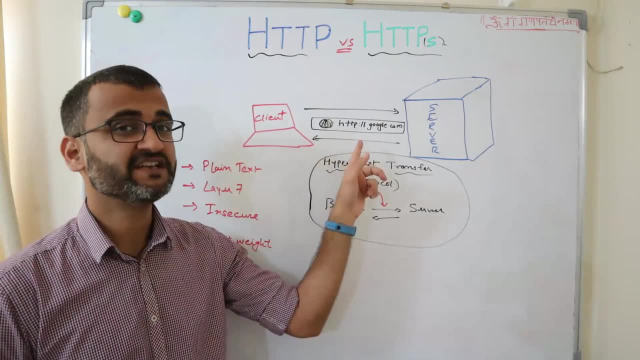 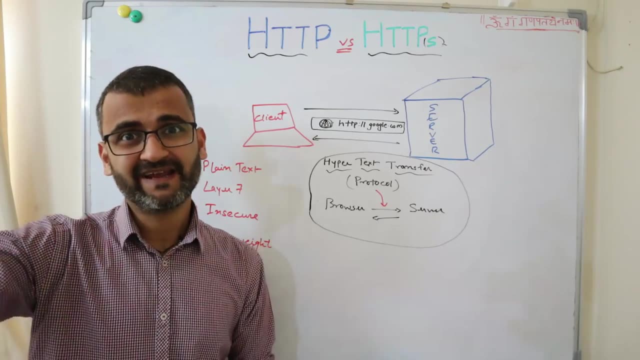 a client is from anothermi, So 가지ya can go to this server and activate the program that allows. Whenever you type anything on your website, for example, if you are typing http//googlecom, then this particular protocol enables you to contact the Google web server and get all. 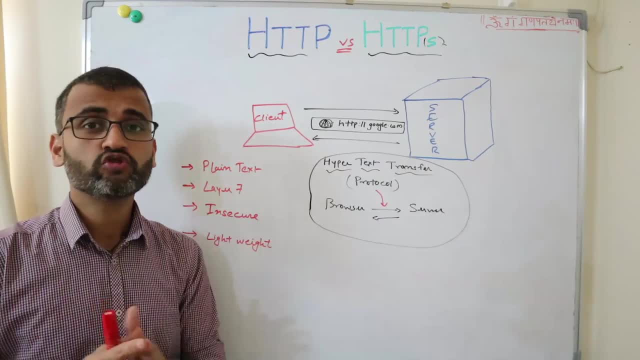 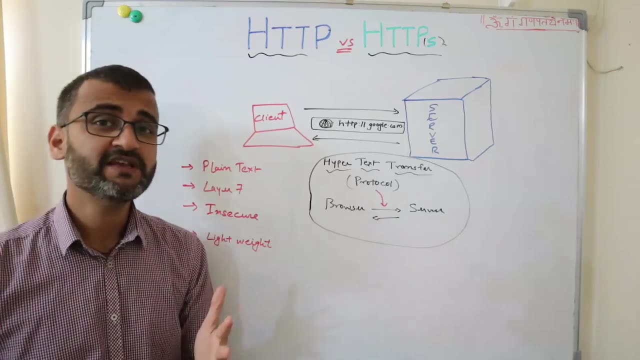 the relevant information from that particular server. So what are the features of HTTP? So, first of all, HTTP sends your data and gets your data in plain text. What does that mean? That means that if you are accessing, maybe, your banking site, for example, although you 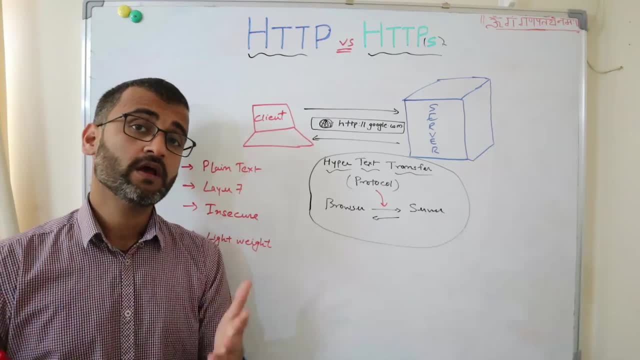 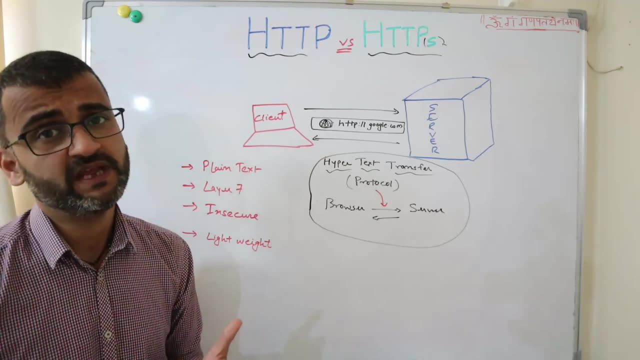 will not be able to do it because it's always secure now. but if suppose you are accessing anything over HTTP, over a public Wi-Fi, there's a very good chance that someone might be sniffing into that particular communication and might get the sensitive data. whatever you are entering, 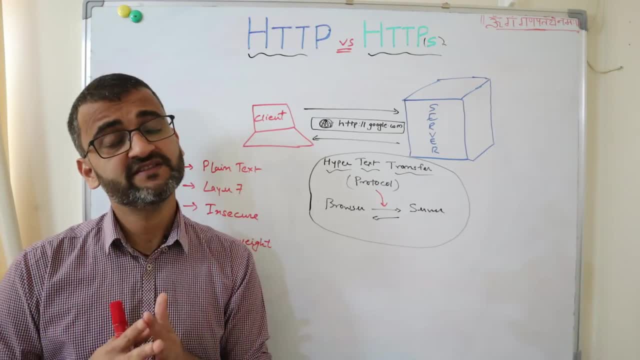 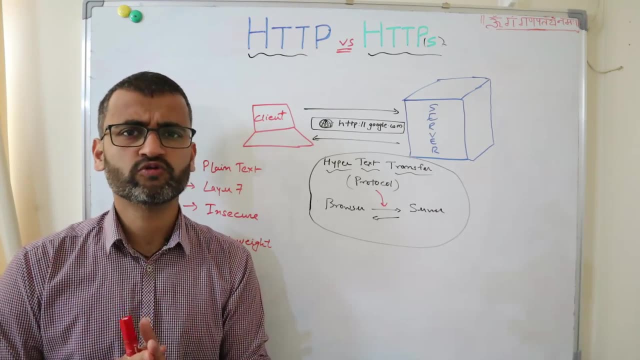 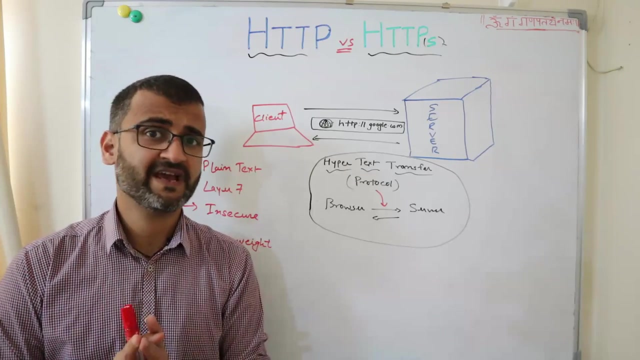 on the browser. So that's why HTTP is very, very insecure and it could be very, very easily hacked. And that's why HTTPS has now come into picture, and almost every website, every company, now has their HTTPS URLs which can be accessed by everyone. 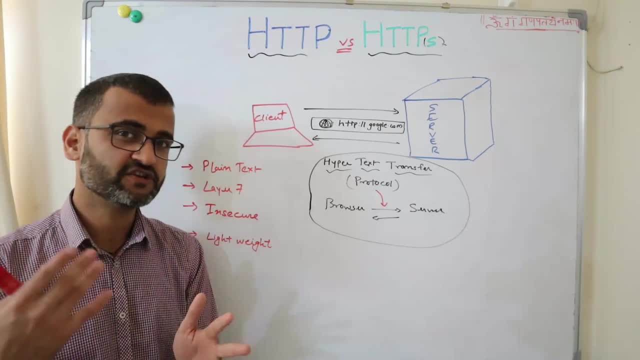 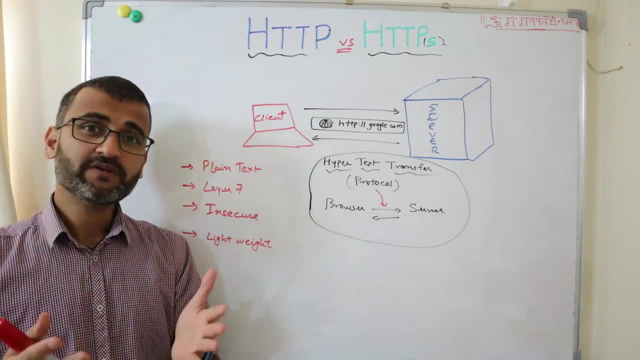 But before we go on to HTTPS, let's first understand some features of HTTP. So first of all, as I said, it sends your data and receives the data in plain text. Then it is a layer seven. So what do we mean by layer seven protocol. 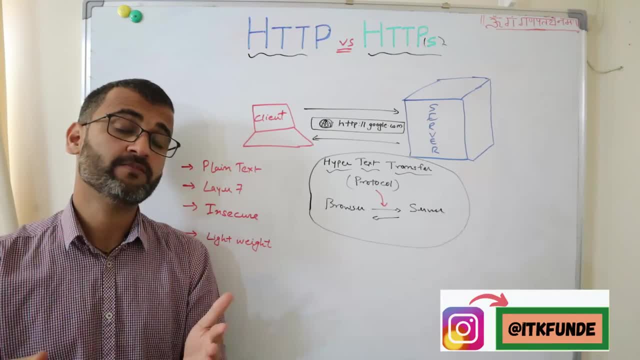 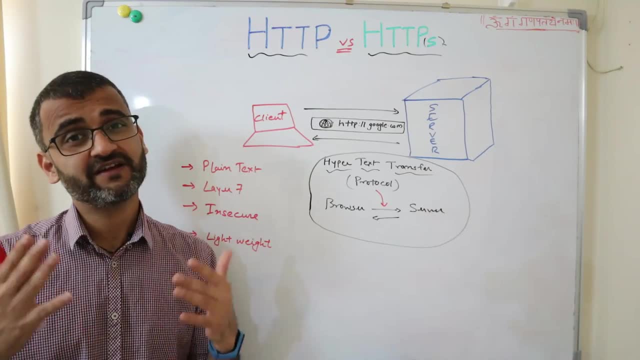 Layer seven protocol. you can understand, if you have understood what is OSI model, what is OSI, what are different OSI layers, the seven layers of OSI model. You can watch that video. I'll give you a quick nugget, which I created for remembering this particular, all the seven. 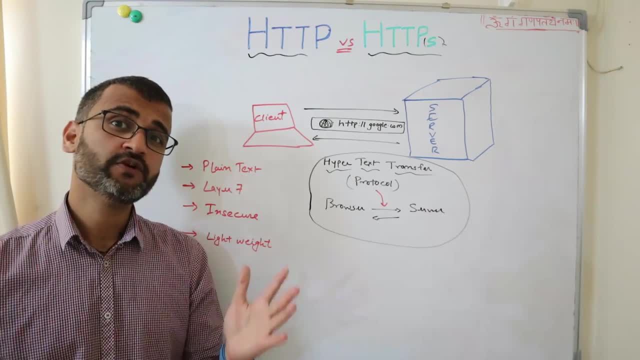 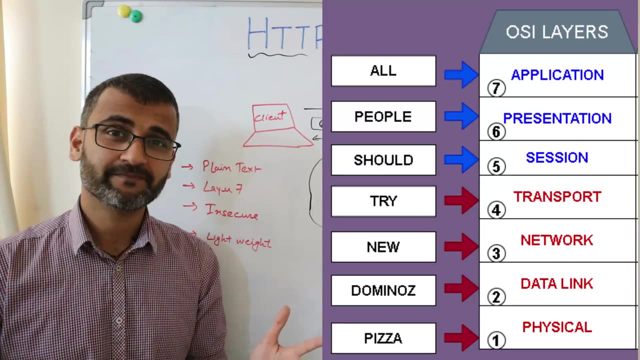 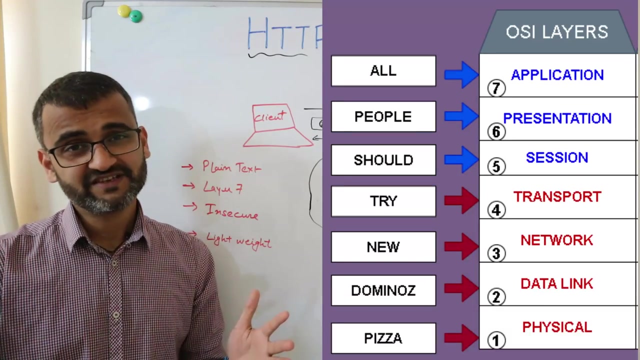 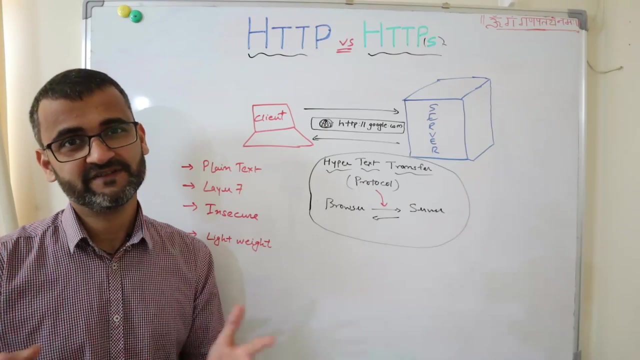 layers of OSI, which is: all people should try new Domino's pizza. All people should try new Domino's pizza. Now you can remember it as application layer, presentation layer, session layer, transport layer, network layer, data link layer and, at the end, the physical layer. 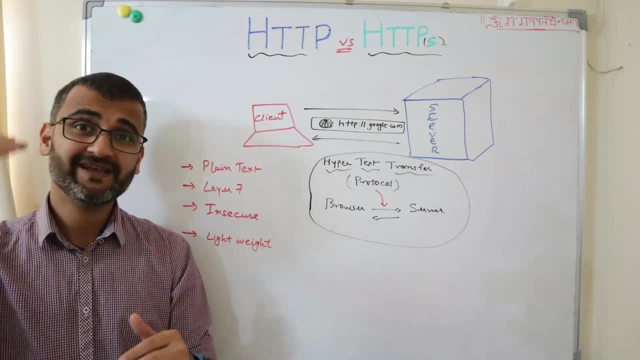 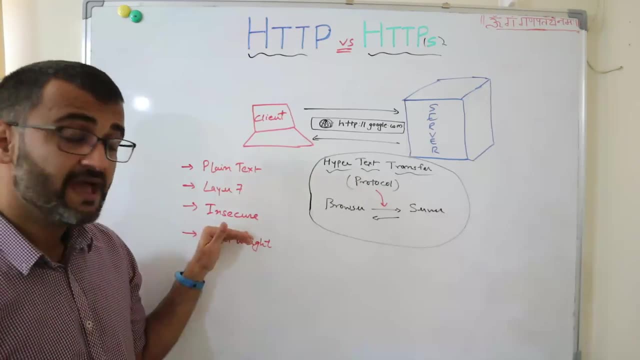 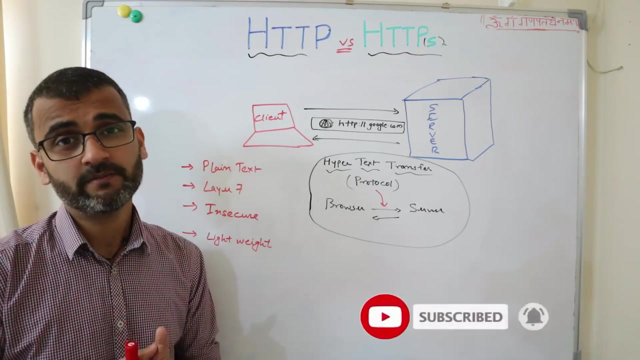 So when I say layer seven, that means that HTTP protocol is right at the top of that particular hierarchy and it resides at the application layer. I also told you that it is very insecure because there is no security in build and everything which we are communicating happens over plain text. 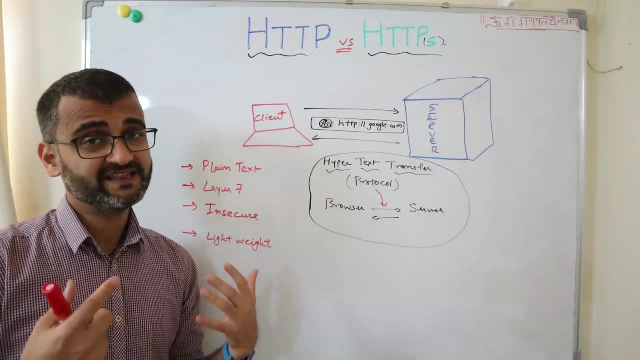 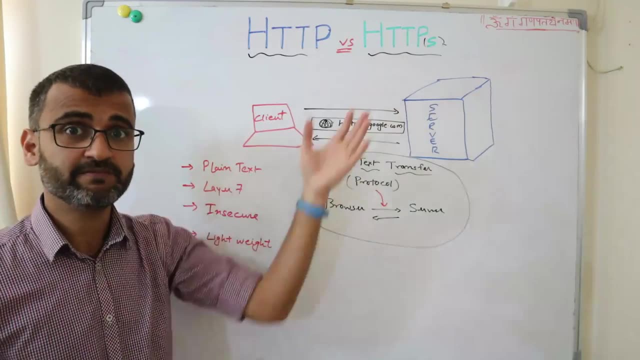 One good thing about HTTP is it is very lightweight and that's why it gives you better performance, because you know you do not have any encryption, What Whatever. You do not have HTTPS, but in HTTP you do not have all those mechanisms to secure the. 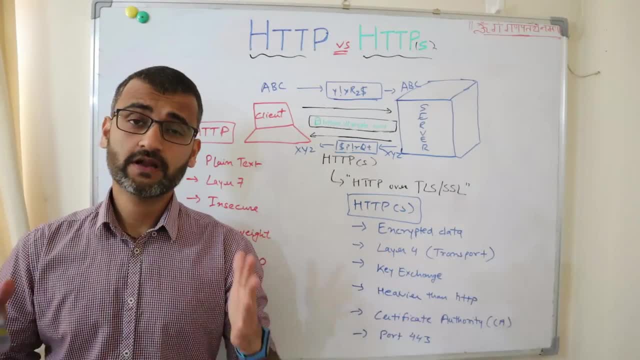 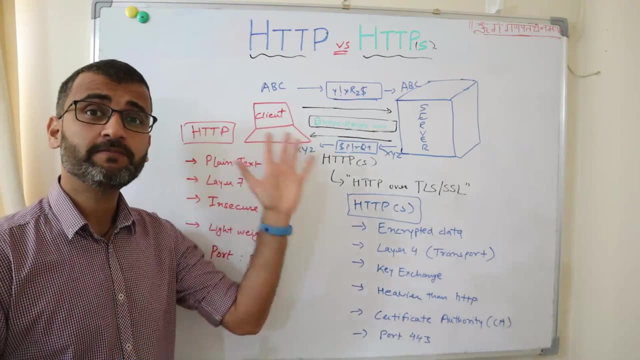 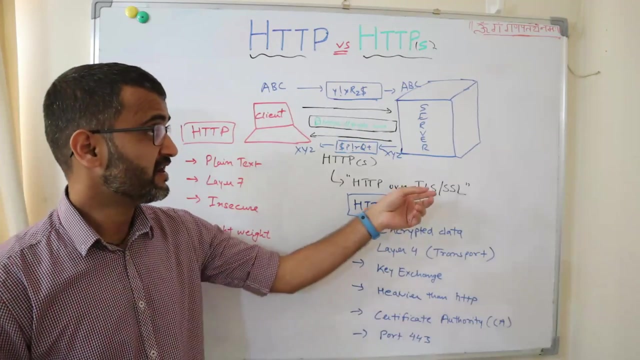 data and that's why the whole protocol is very lightweight. So, friends, now let's understand what is HTTPS and how it is more secure than HTTP. So, when you are talking through HTTPS, you have an additional layer of security which is provided through SSL or TLS protocol, which is transport layer security or secure socket. 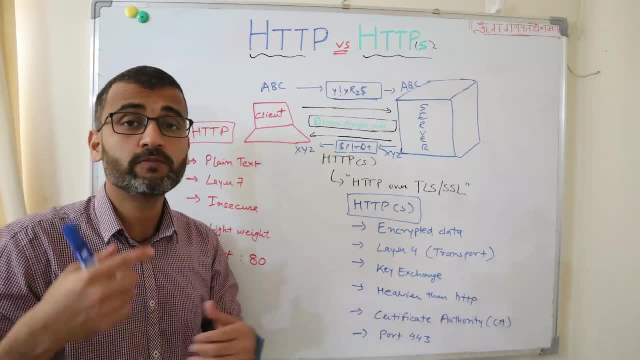 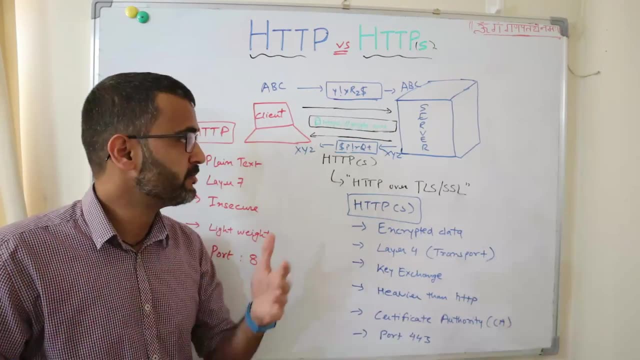 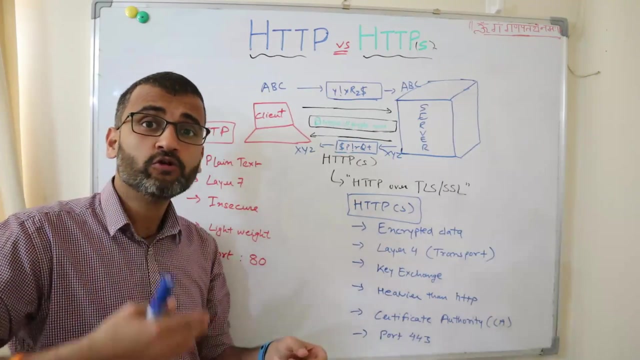 layer, Secure socket layer, was the previous versions of this protocol, but now the later versions are TLS, But these two terms are used interchangeably, So always remember that HTTPS- you can consider it a younger cousin of HTTP, with an overlay of TLS or SSL protocol. 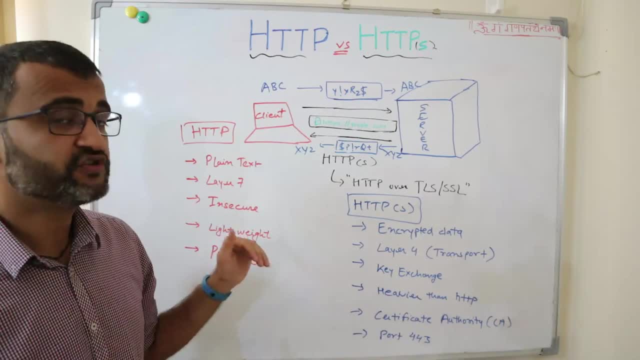 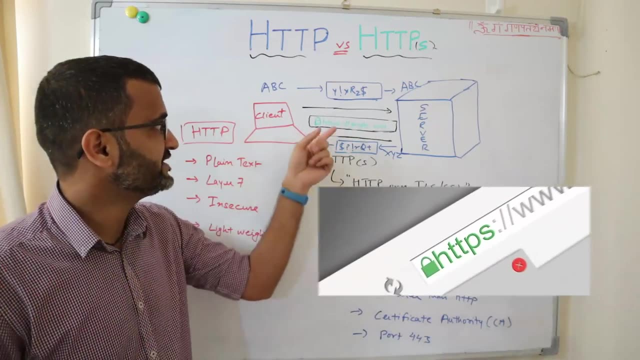 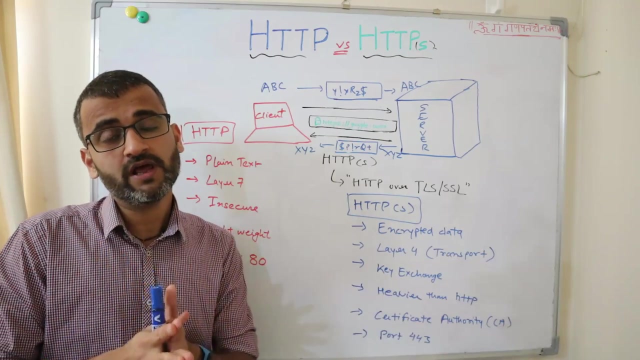 So how exactly it works. So in HTTPS, first thing which you will notice whenever you are opening a bank website, or maybe any any good website which needs to be secured, you will always see a green padlock on the browser. That itself indicates that now you are entering HTTPS, you know protocol and through that, 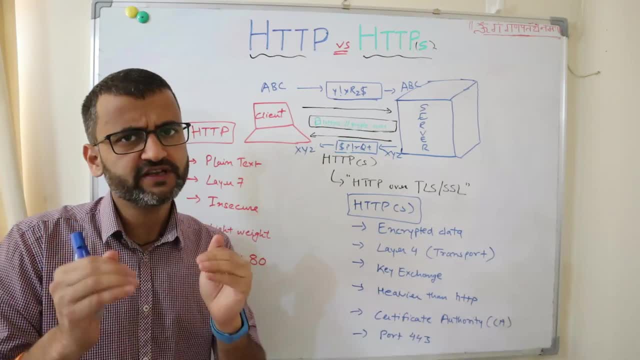 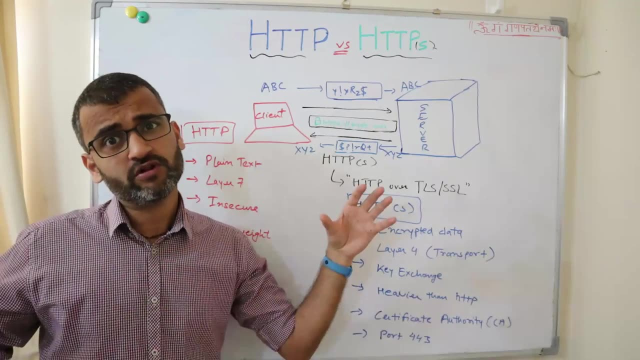 you are entering into a secure communication channel. How it is secure? Because now the data is not going through plain text, it is getting encrypted and decrypted And while it is on the network, you know, no one can could see through what exactly. 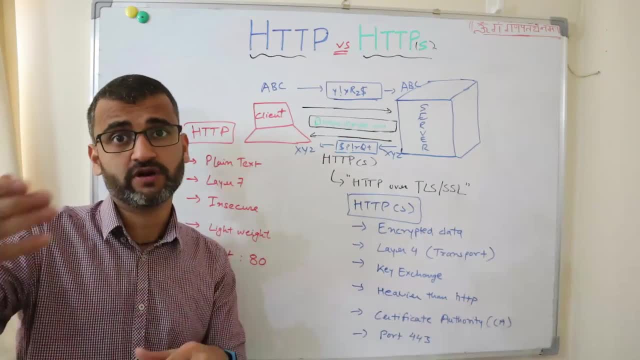 is happening or what exactly you are. you have sent the information or what you are getting from the server. So suppose you send an information like ABC, Then it will. you know it will be sent to the server. So you can see the data. 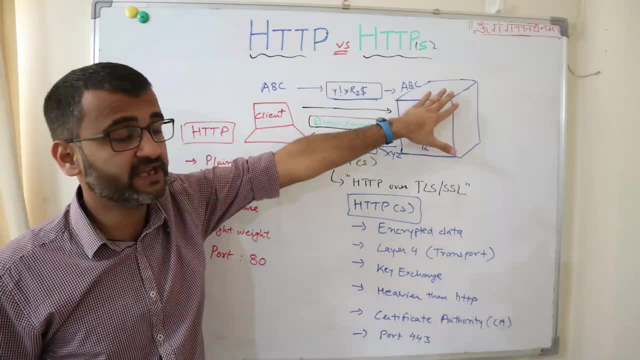 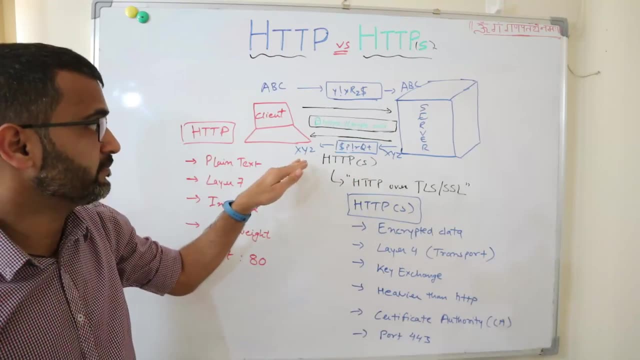 So you can see the data You know get encrypted while on the network and then it will be decrypted on the server side And when server responds with a reply of XYZ, again it is encrypted and decrypted. So someone who's sitting here trying to, you know, do some sniffing on this particular. 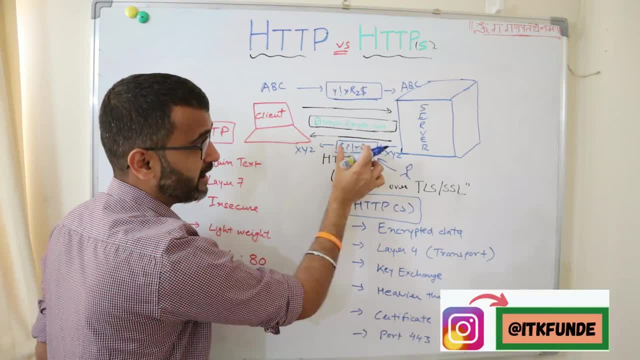 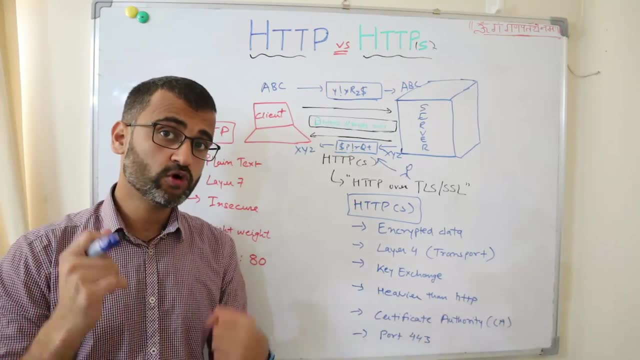 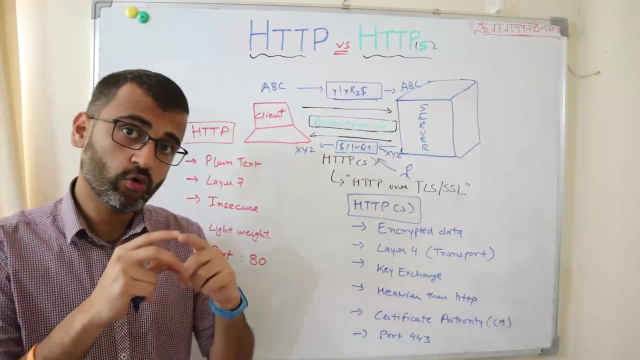 network, then this particular person won't be able to understand what is being sent, Although he will understand which particular server you are targeting, which port you are listening to, what amount of data, The size of the data or the duration, with duration for which you are, you know, opening. 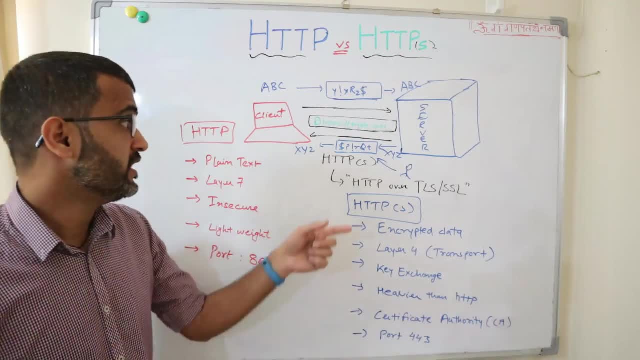 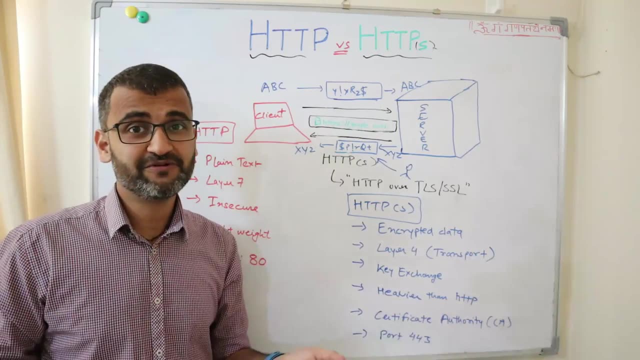 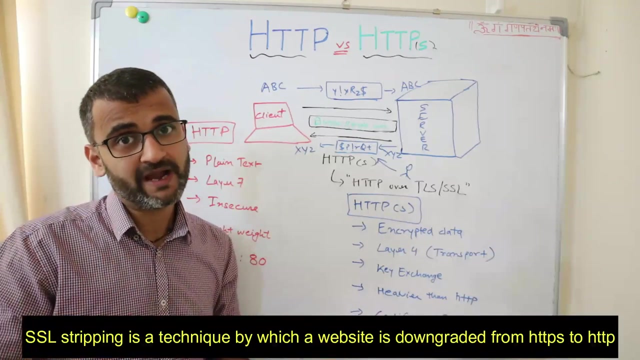 that channel all that information he can still get, but he will not be able to understand or decrypt this particular data which is sent again. you can hack pretty much everything today, So there is a concept like SSL stripping wherein you know you might, you know it. 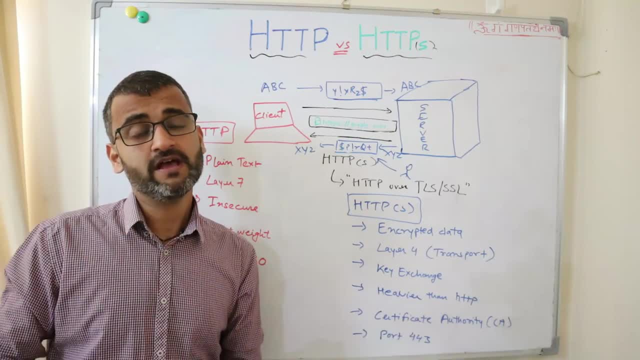 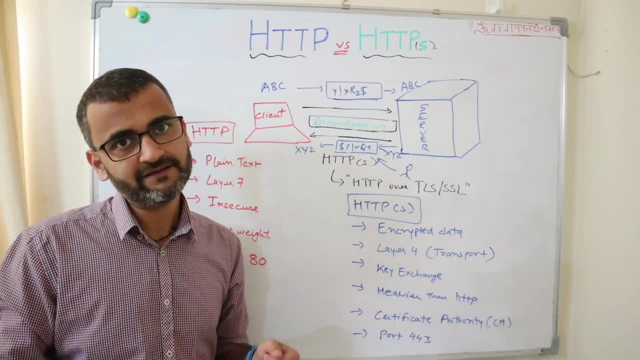 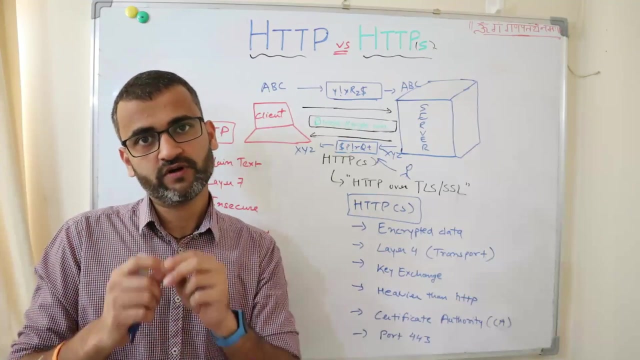 might indicate to you that you are entering HTTPS, but then, using SSL stripping, you might be redirected to a HTTP page. So there are various ways to hack things, but you know, as per HTTPS protocol, if you- you know- send any information over the network, it is very, very secure compared to your. 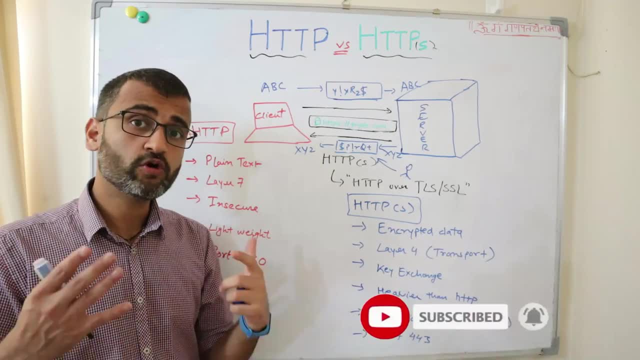 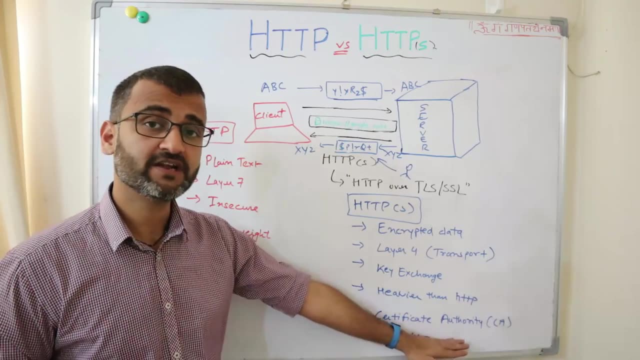 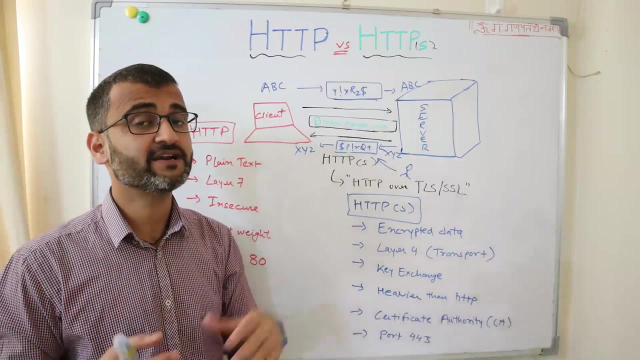 it's HTTP cousin and how it becomes secure because it uses SSL certificate. And these SSL certificates are, you know, are signed through a certificate authority and that particular certificate authority- Okay, You know- is installed on the browser. browser should understand that. okay, this is a legitimate. 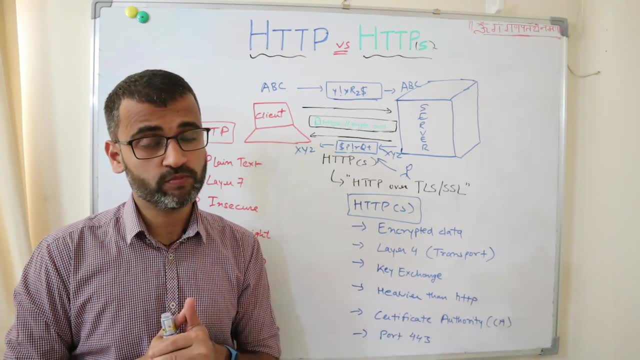 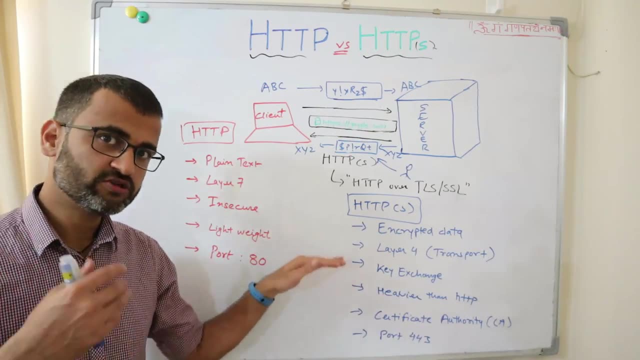 certificate and only then that communication channel is open. So we'll understand for encryption in more detail in a while, but just run through. let's run through some features of HTTPS. So first of all, as I said, it encrypts data using SSL or TLS protocol. 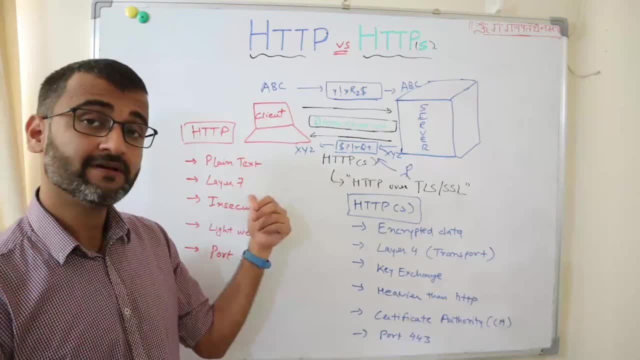 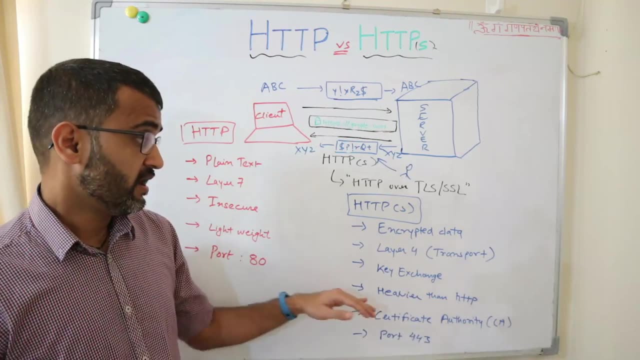 Then it is a layer four, transport layer protocol, unlike a layer seven of HTTP. Then there is a public and private key exchange For encrypting and decrypting data. it is heavier than HTTP. So obviously, when you are adding more layer of security, when you're adding, you know, 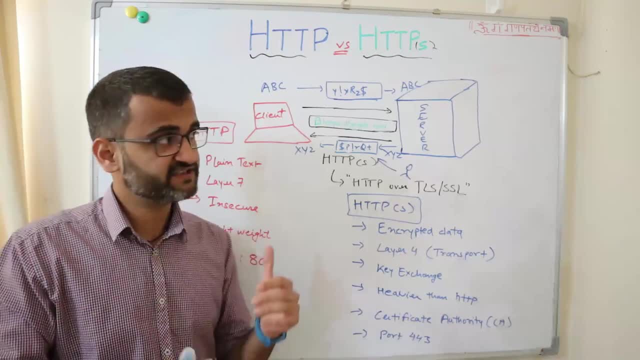 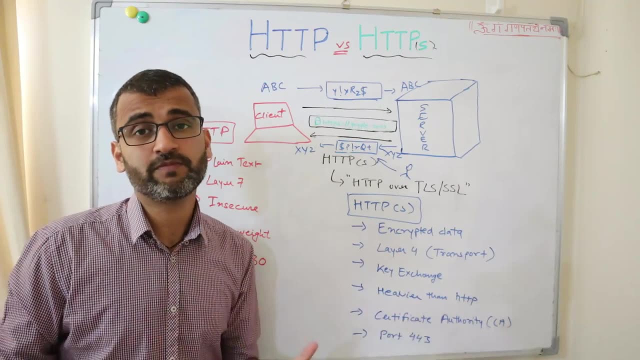 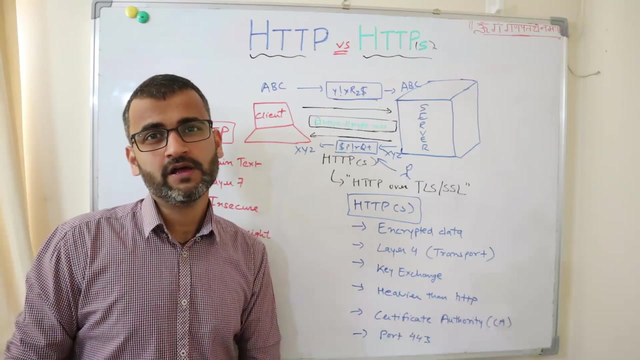 more additional encryption, decryption onto this particular HTTP protocol. it's it is tend to be become heavier. So if you are looking for very good performance, then you know there is some sometimes you know the websites which are non-critical, which hosts non-critical data, then those 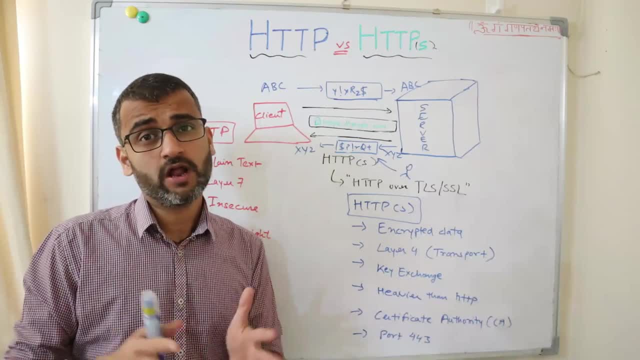 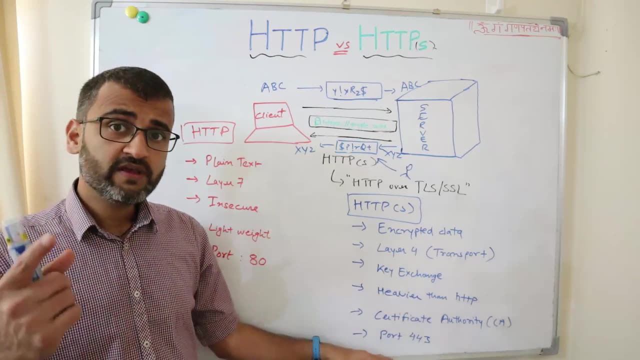 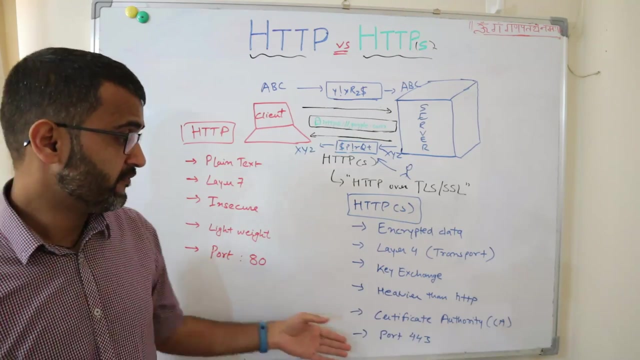 websites might redirect you to HTTP protocol, but still now, more and more, all the websites are encouraged to go only via HTTPS. Then one thing which I missed previously was the default port. The default port on which HTTP protocol listens to is port 80 on any server, while for HTTPS, 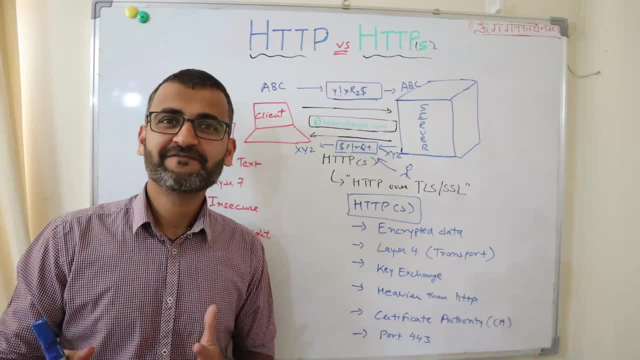 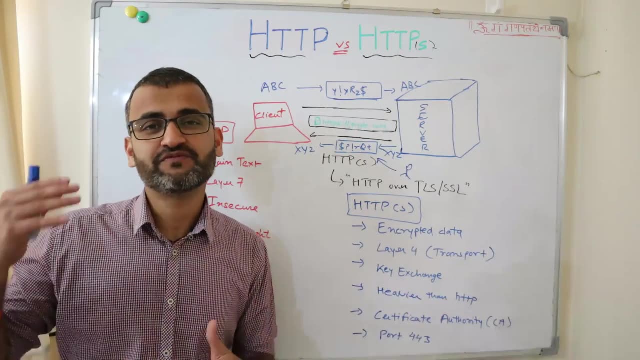 it is port 443.. So, friends, let's take a real life example to understand how encryption and decryption exactly works. Suppose we are in 1970s or 60s, When there is only letters to share your feelings with each other. 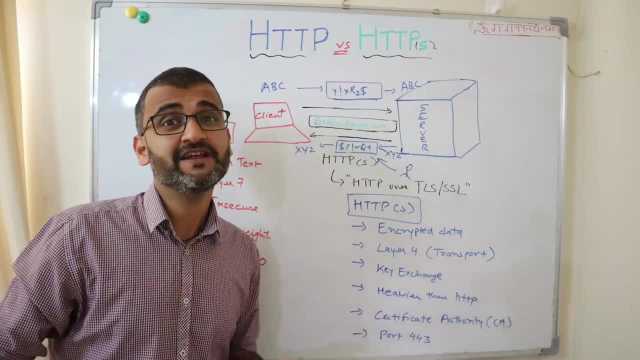 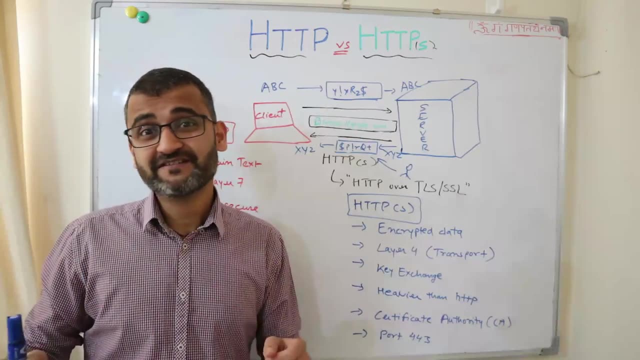 And there is this boy, Trevor, who wants to share his feelings to Maria, but at the same time he wants only Maria to understand what he's writing. And he writes in a letter four lines, And those four lines were not a direct proposal. 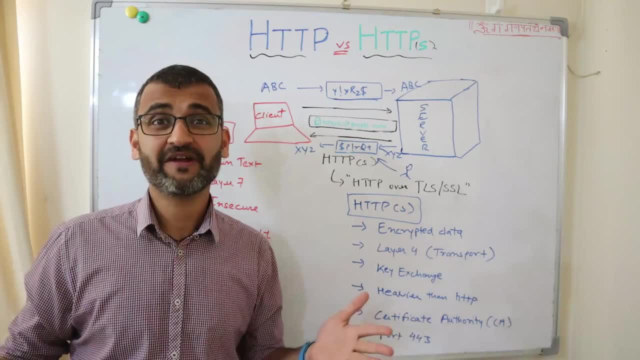 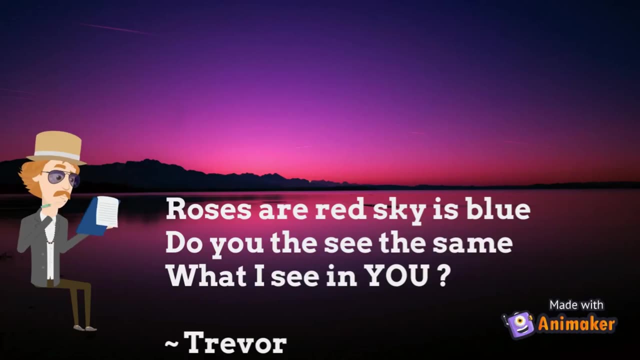 It was an indirect, encrypted message for Maria. He writes: roses are red, sky is blue. do you see the same what I see in you? And when this letter goes to Maria, Maria decodes it, decrypts it and writes back replies. 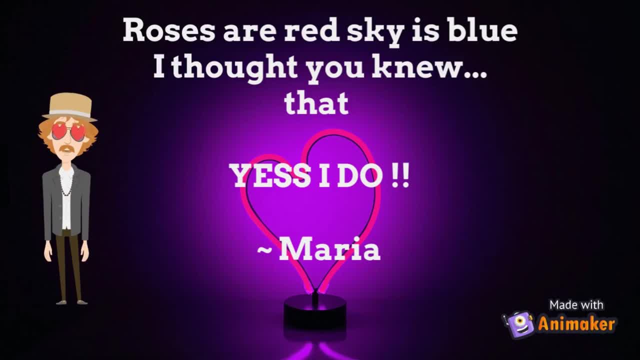 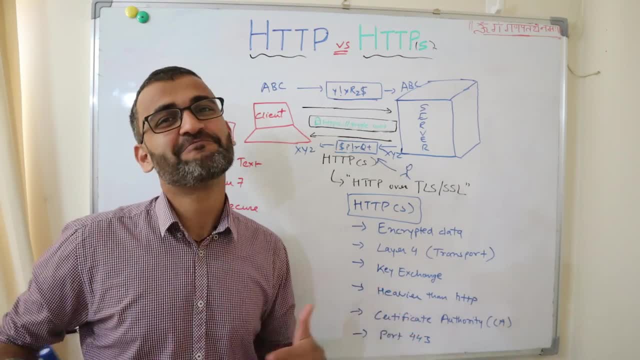 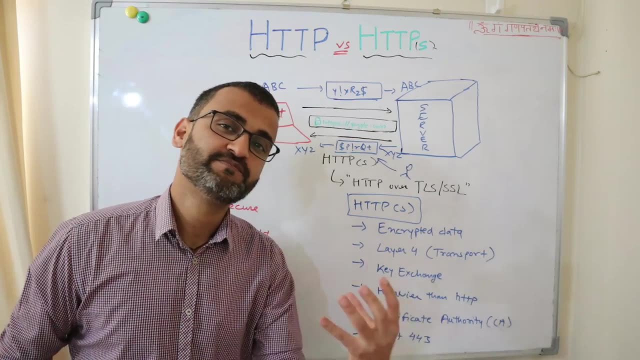 back And Maria replies: roses are red, sky is blue. I thought you knew that. yes, I do. So this is encryption and decryption, guys, in a more loving way, right? So, similarly, when you are doing encryption and decryption, there is some message which 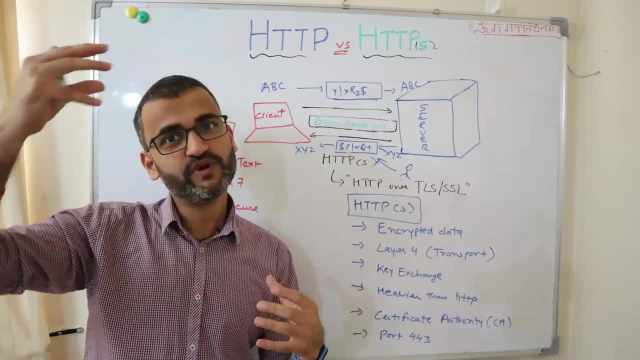 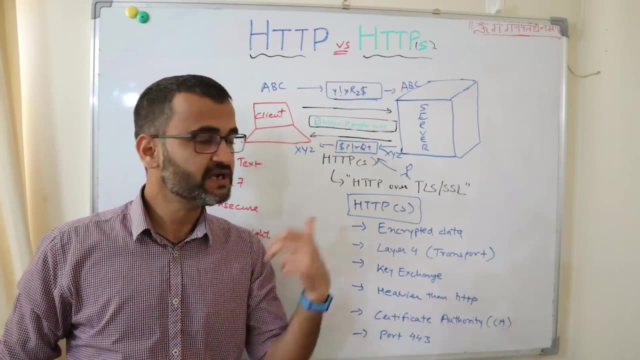 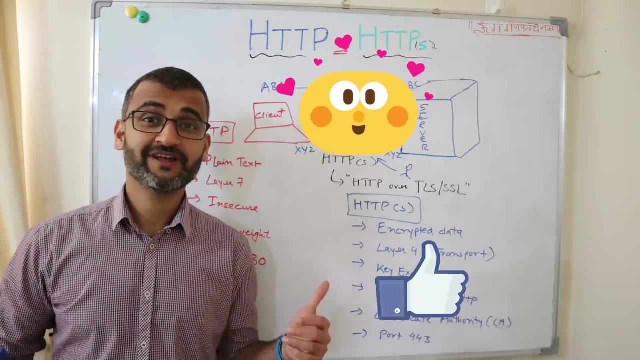 is being sent and only the server with which that particular message can be decoded is decoded to can decode that message. Now how it happens through SSL encryption, we'll understand with the help of yet another example. So, friends, if you don't like the tutorial, at least hit the like for the poetry I've. 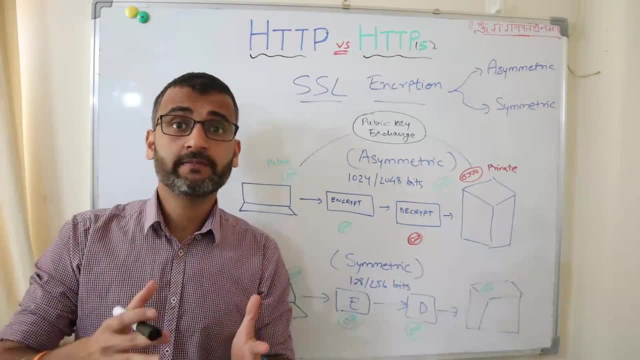 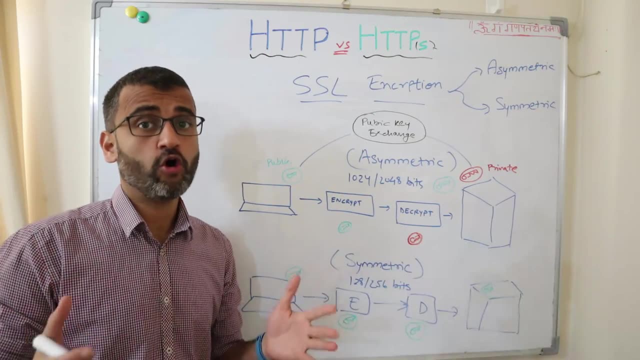 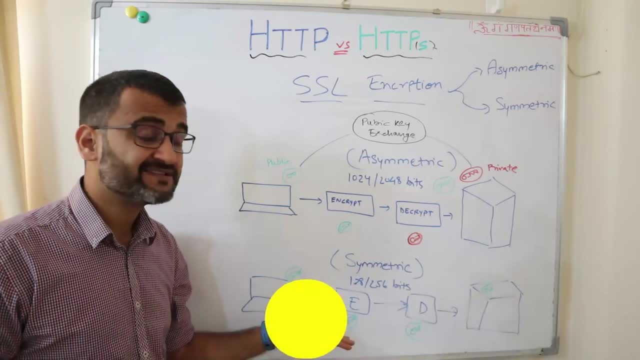 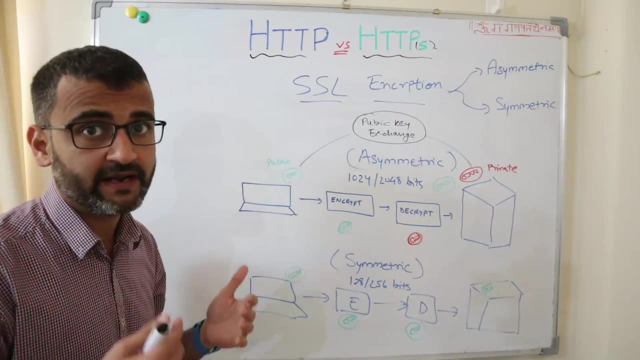 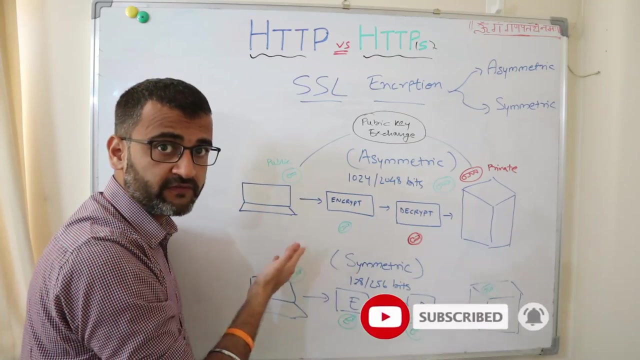 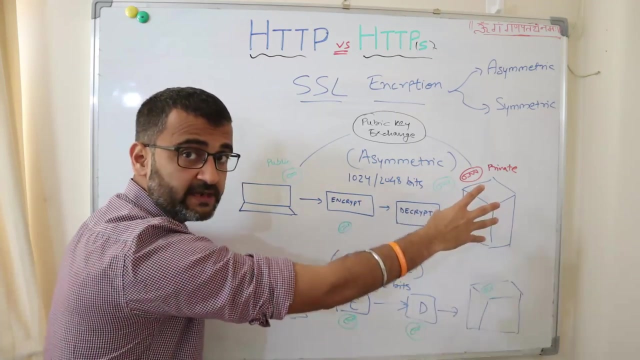 is a mobile kind of, let's say, neural library. that's not all, or rather a drive Internet from the current service. If you don't want a SCIMMATRIS sp suit, let's say, let's say, let's say it's based on. 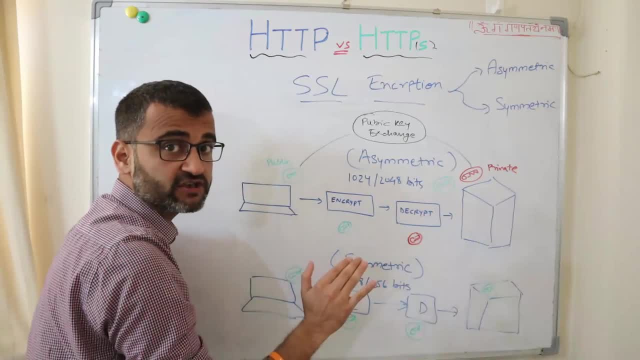 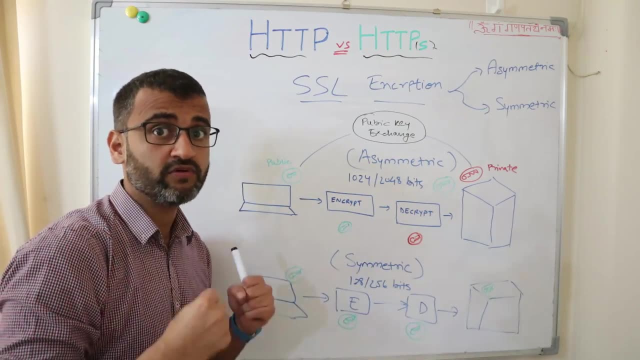 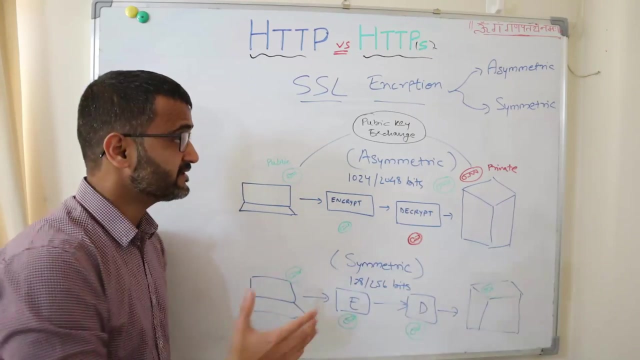 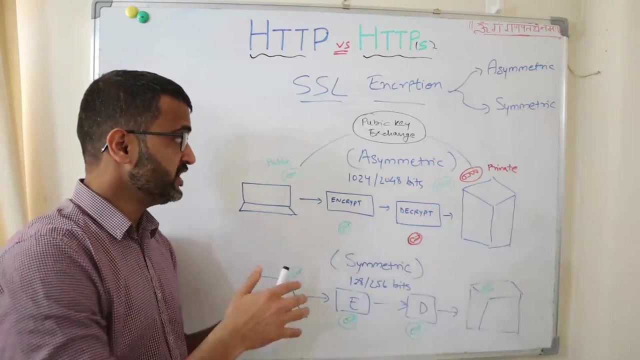 SSL decryption keys only with this particular server. no one else has it. so that's why asymmetric encryption is more stronger and more tougher to crack, because it has two different keys working together to secure the data. now, that's why the size of this particular encryption is of 1024 and 2048 bits, because you 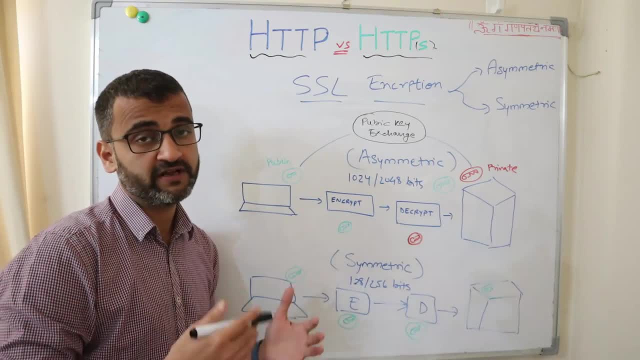 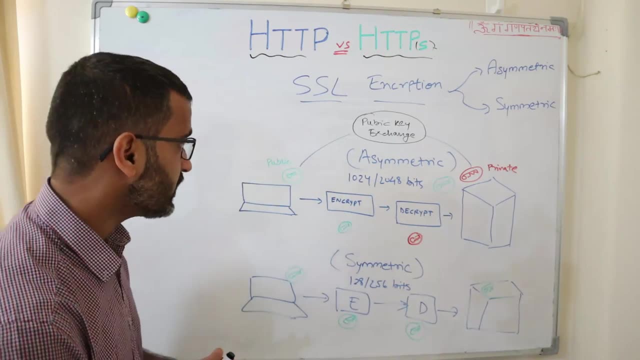 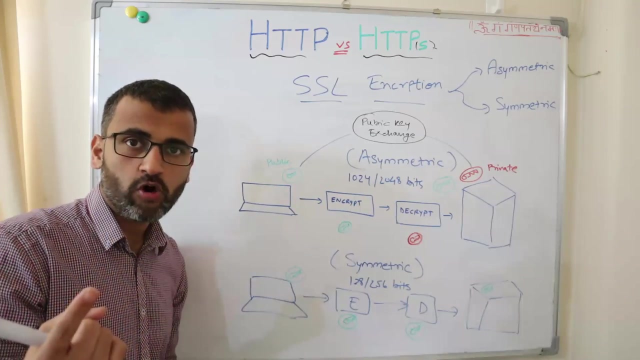 need to maintain a public key and the private key separately to encrypt and decrypt the data. so this is asymmetric encryption. in symmetric encryption, it is a simpler form of encryption wherein you have only one key and that one common key is given to the client and the same key is. 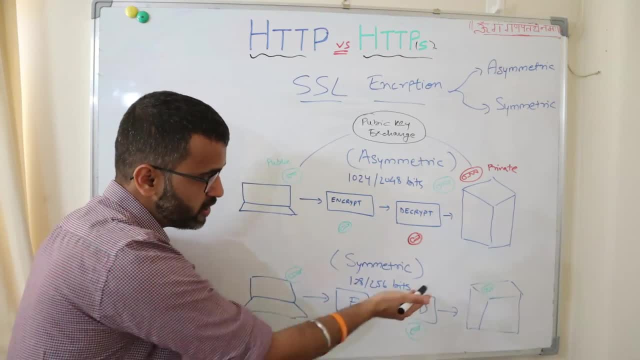 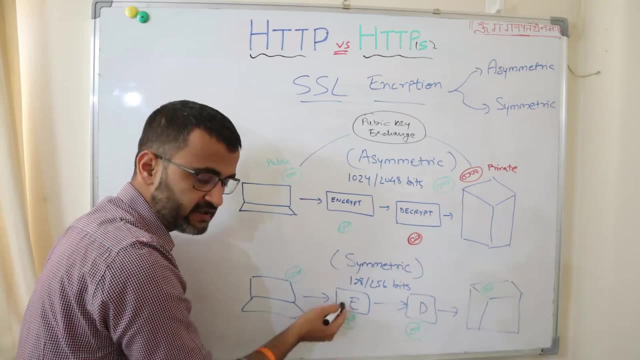 used by the server for decryption of the data. so the this particular common key will be given to the you know client and then, using this key only, the encryption will happen and the same key will be used for decryption of the data. so this is a simple form of encryption where you have only one. 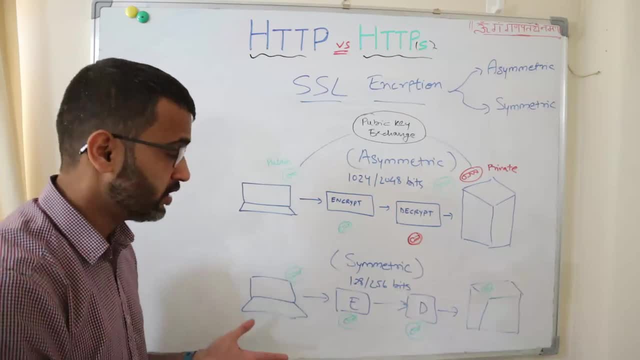 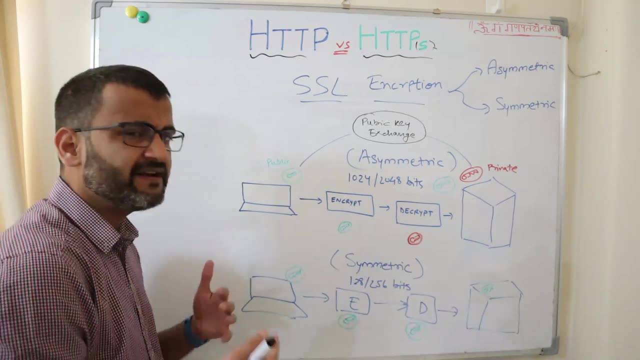 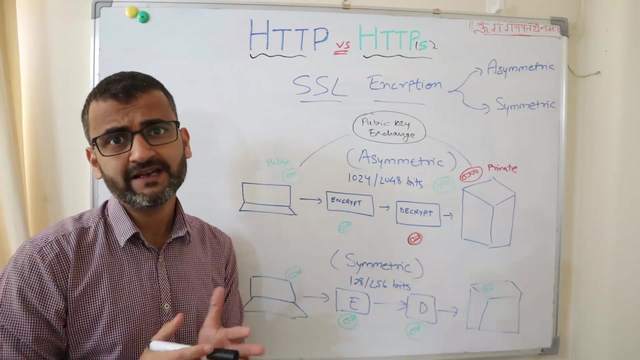 encryption. so again, this is a simpler way to, you know, encrypt and decrypt the data and that's why it is lightweight. it is only 128 and 256 bits and relatively easier to break, but by no means it is less useful. so whenever you are doing ssl encryption generally we combine asymmetric and 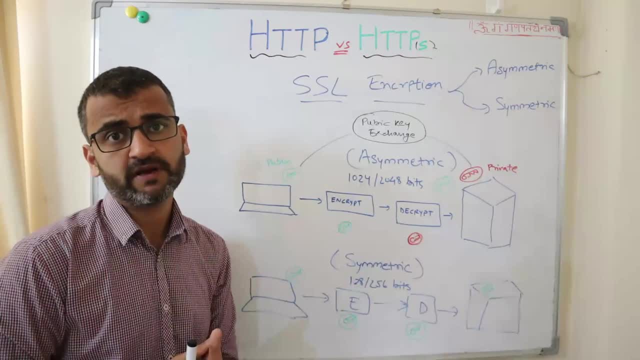 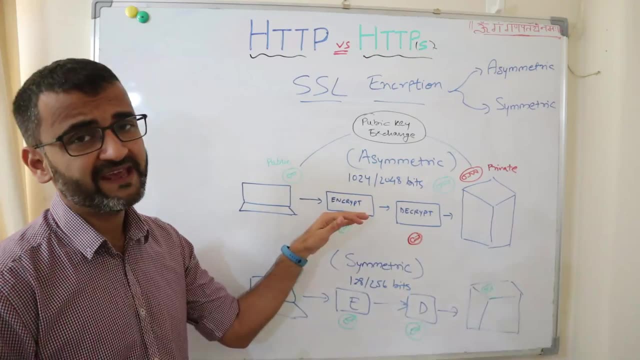 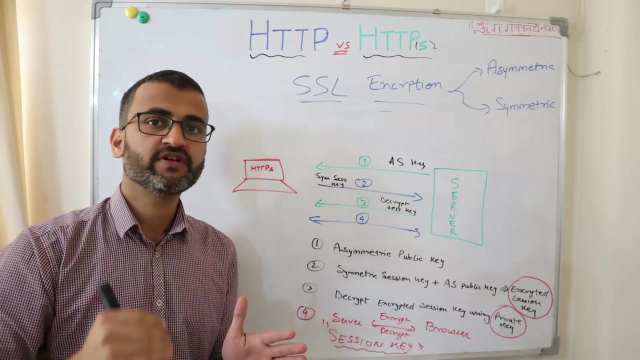 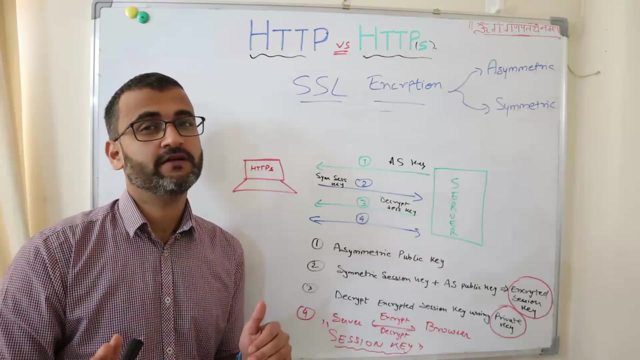 symmetric together and then the whole communication becomes quite robust and secure. so now let's understand how this whole communication flow happens using asymmetric and symmetric encryption decryption. so, friends, now let's understand how ssl encryption works using symmetric and asymmetric keys. please pay attention, because it might be slightly confusing. i'll try to explain it slowly. 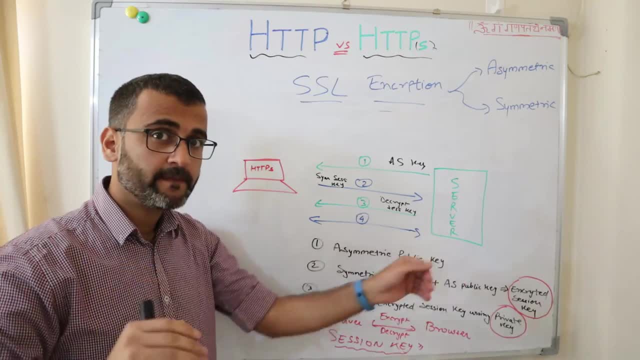 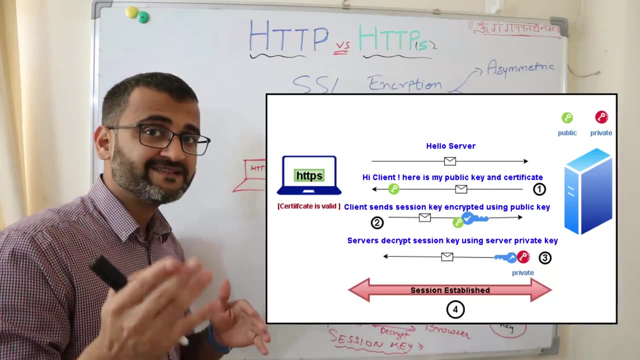 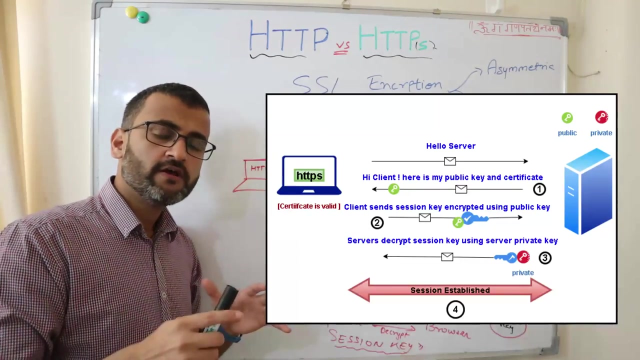 just try to understand. okay, so in step one, the server will send over the asymmetric public key to the browser. you, as i said, asymmetric keys, has public key and the private key, so the public key will be sent to the browser. now, browser will generate a symmetric session key. now, as i said, symmetric encryption. 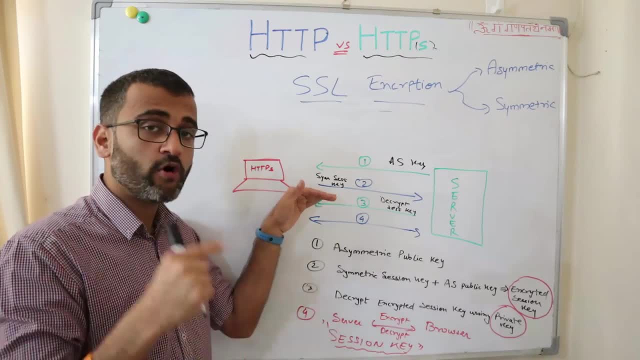 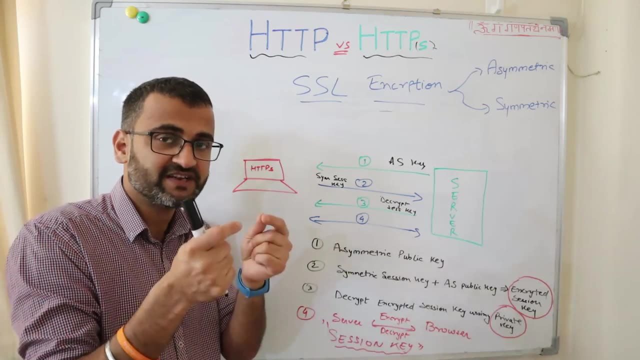 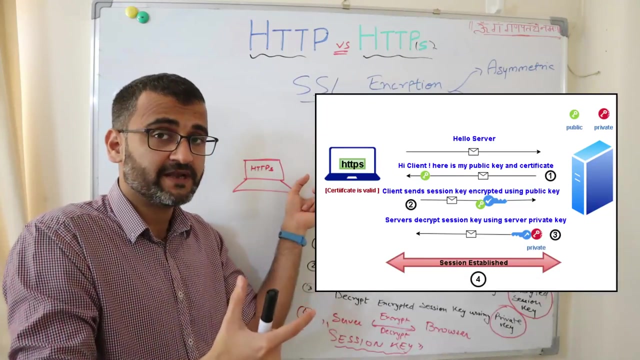 only has single key. okay for the server and the client. so now what browser will do? browser will generate a local session key, symmetric encrypt, encryption based session key, and it will encrypt it because this session key will be, you know, a generic key. how it will be encrypted? so it will use the public, asymmetric public key which was given in step one, combined. 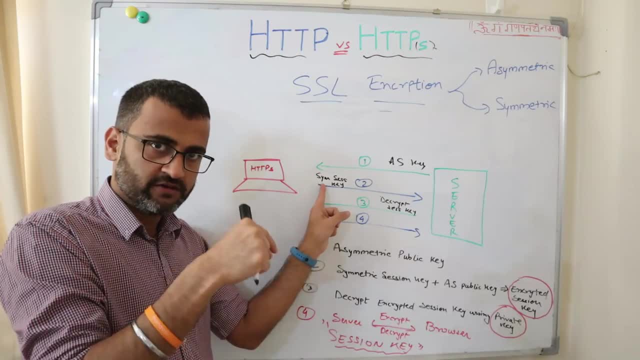 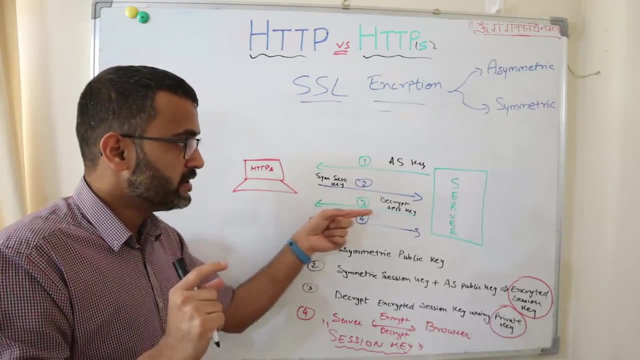 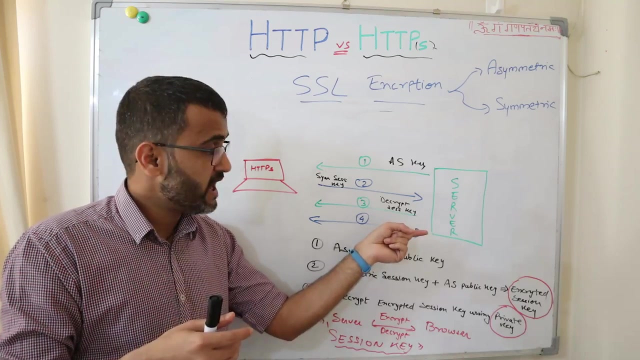 it with the locally generated- uh you know- session key and then encrypt this particular key and send it in step two to the server. now, in step three, server will take that particular uh you know key which has come in and how it will now decrypt it. now this particular browser has used the public 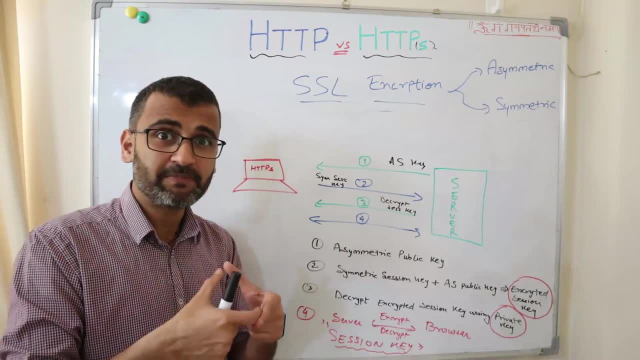 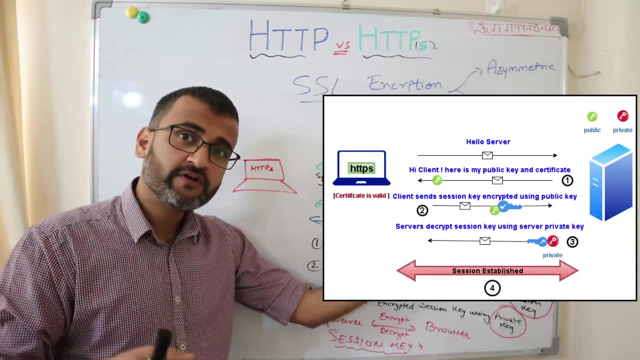 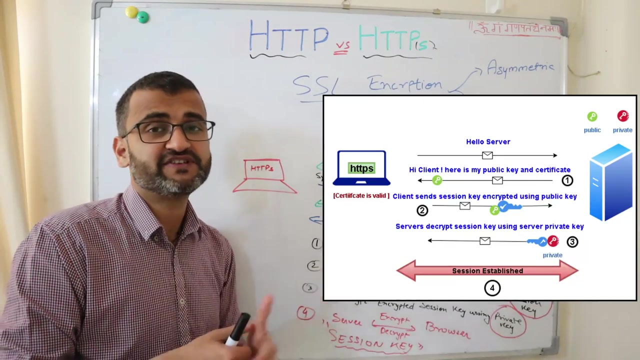 key, but the server will use the private key to decrypt the encrypted session key which has come to um, you know to it. so now this particular server will use the private key- asymmetric private key- to decrypt the session key which has come in. so in step three, once this particular decryption, 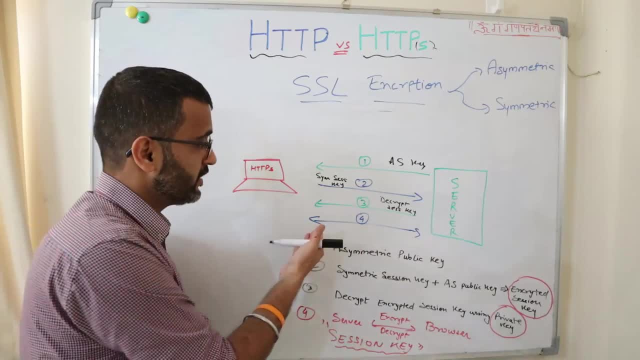 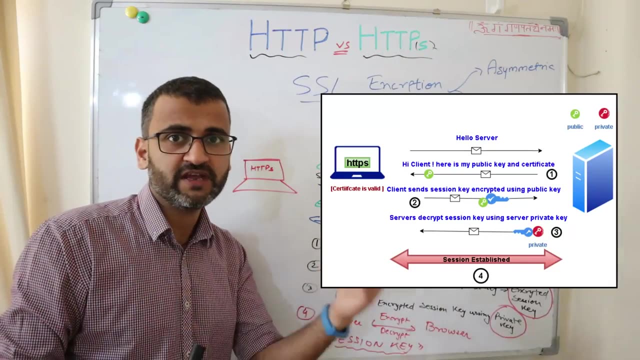 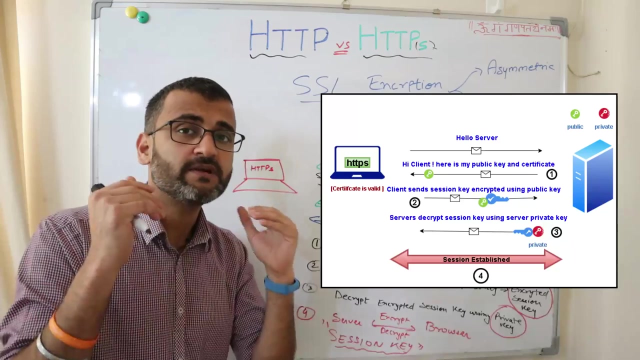 happens from step four onwards. the server, the browser and the server can communicate using that that particular session key, using encryption and decryption of that particular session key, And that particular session key will last only for that particular session. If you close the browser or if you log in the next day, then you have to run through. 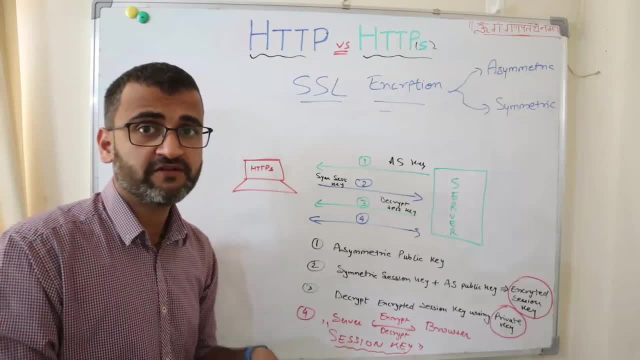 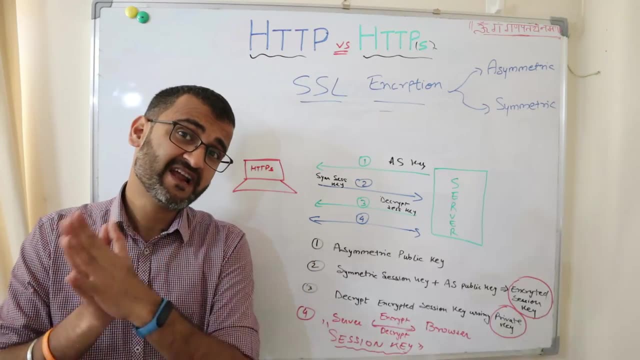 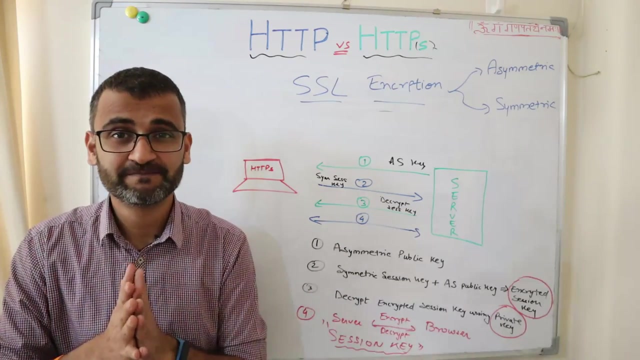 this whole communication channel. again and again, the session key will be created. So, friends, I hope you now know a bit more about HTTP, STTPS, what S stands for in STTPS, how it is more secure, how encryption- decryption- works using symmetric and asymmetric keys. 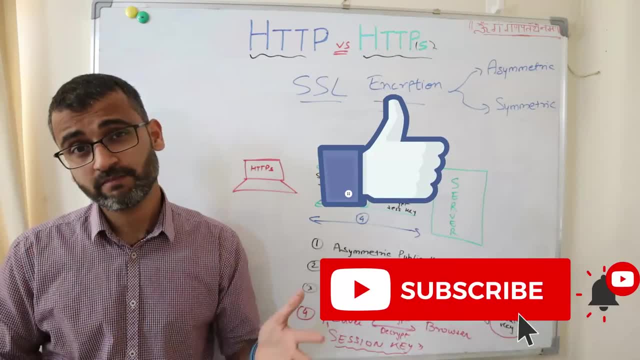 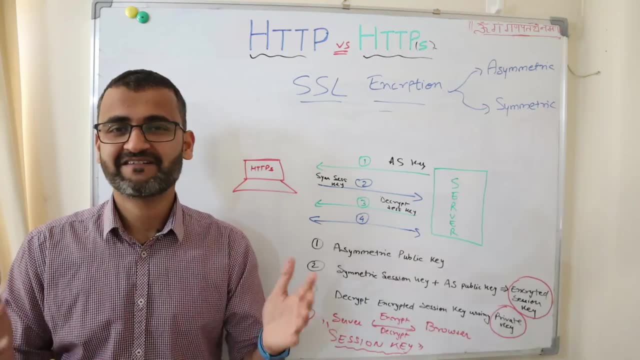 So, if you did, please hit the like button, hit the subscribe button and the bell icon so you exactly know when I upload my next video. Let me know in the comment section what you would want to learn next. I try to make videos in best of my capacities. whatever I know, I try to share with you all. 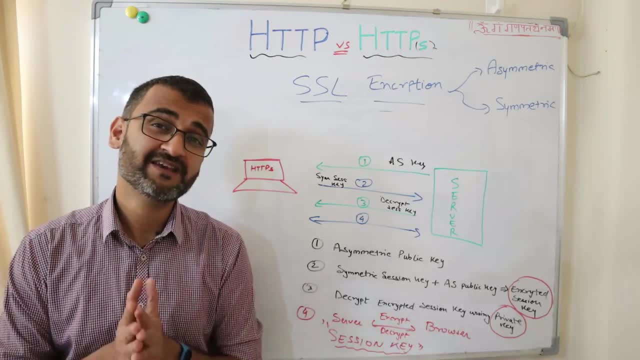 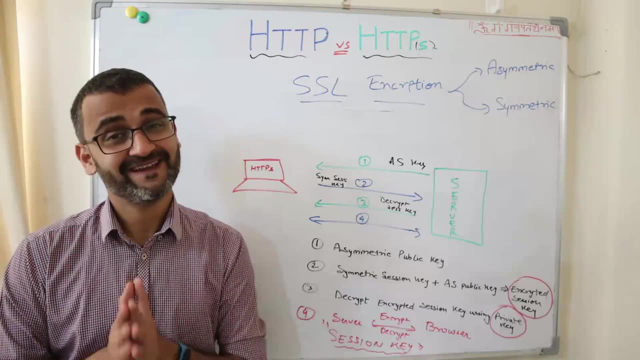 So, yes, do let me know what you would want to learn next, and if I know anything about it, I'll be more than happy to share with you all. So until next time, Please keep learning, guys, keep growing and, yes, keep hustling. Bye for now.